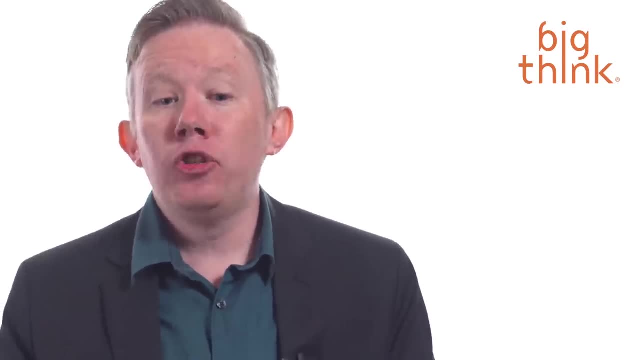 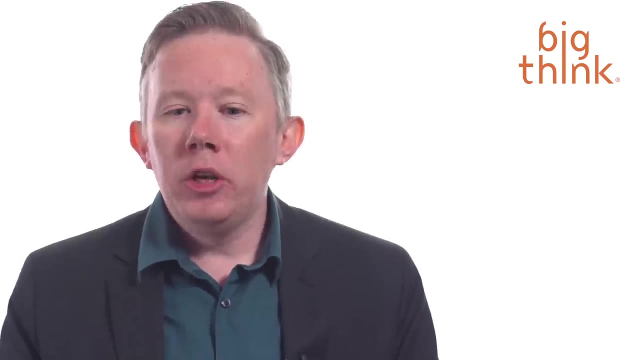 Game theorists call this a mixed strategy, in order to make sure that your opponent can't get the leg up on you. The nice thing about these random strategies is that they ensure that your opponent can never outthink you, So even if you think your opponent's a little smarter than you or a little bit more sophisticated- 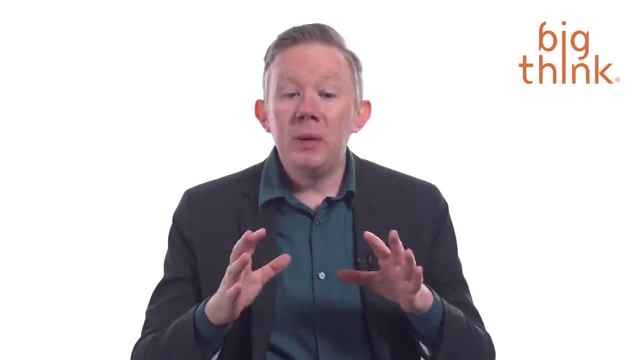 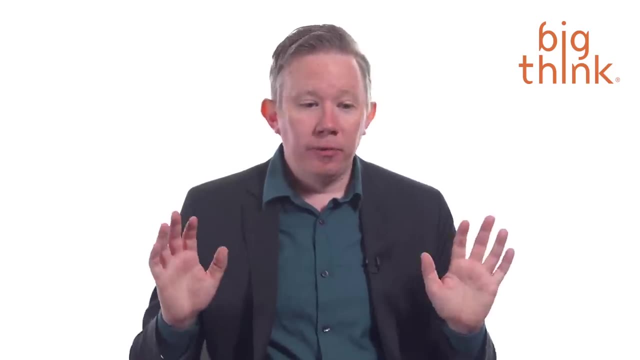 than you or has a little bit more information than you do. the fact that you're being random to a certain extent means that they can't outthink you. Now how do you figure out how to be random? I'm not saying just flip a coin all the time or whatever. 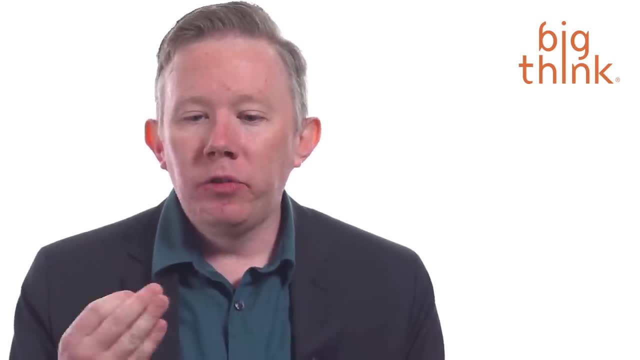 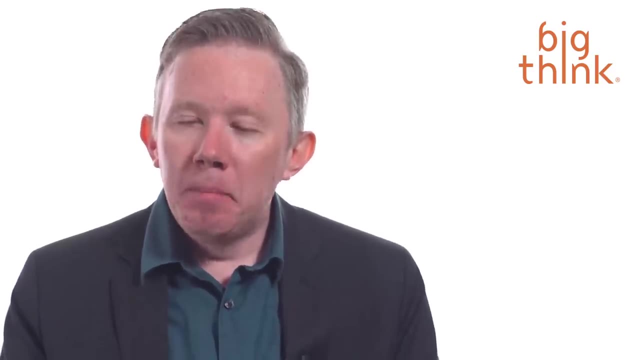 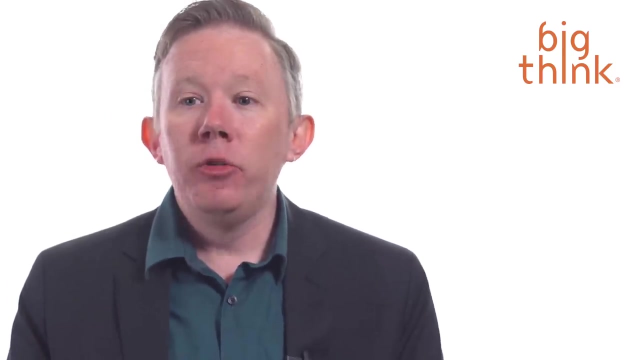 What game theorists have figured out is that in zero-sum games, the best strategy to pursue when you're against a sophisticated opponent is to adopt the strategy which minimizes your maximum loss. This is sometimes called the mini-max strategy. So the idea is: you think what's the worst case scenario for me? 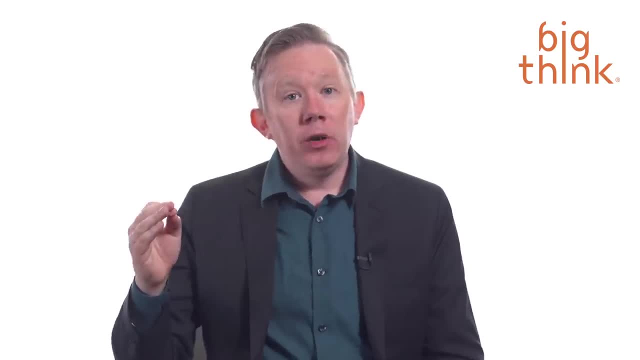 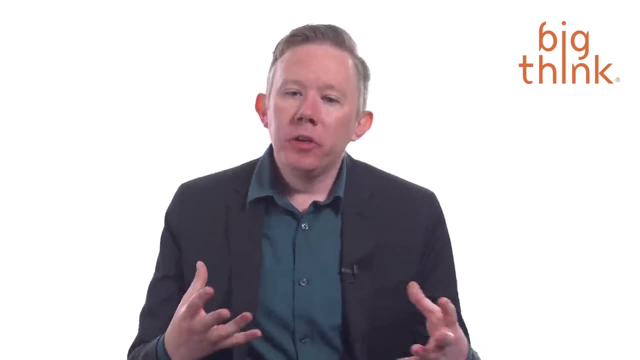 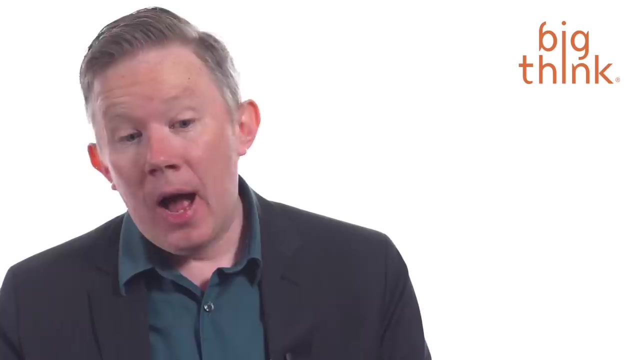 What could my opponent do that would make me worse off, And then you figure out what's the best strategy against that, So you're minimizing your maximum loss. Game theorists prove that if you use this way of thinking- minimizing your maximum loss- you ensure that, no matter how sophisticated your opponent is, you've guarded against the 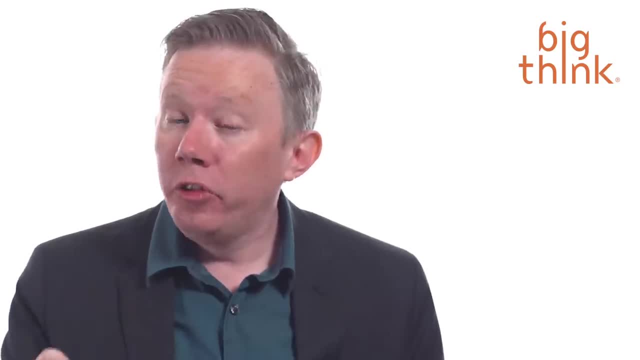 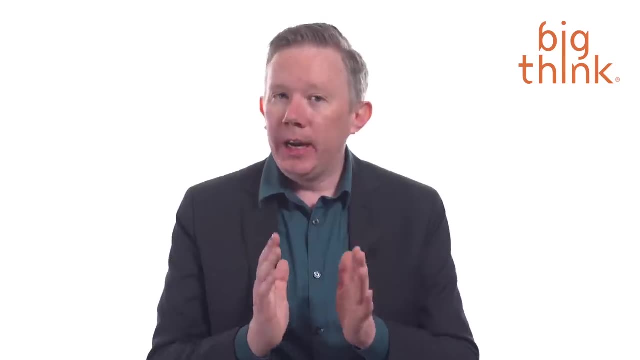 worst case scenario. And not only that, but in zero-sum games You've done the best you can possibly do. That's not true in games that aren't zero-sum. So one has to be very careful about employing this strategy, because if you're mistaken and 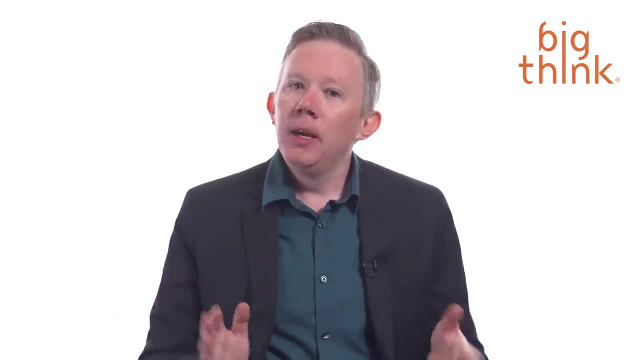 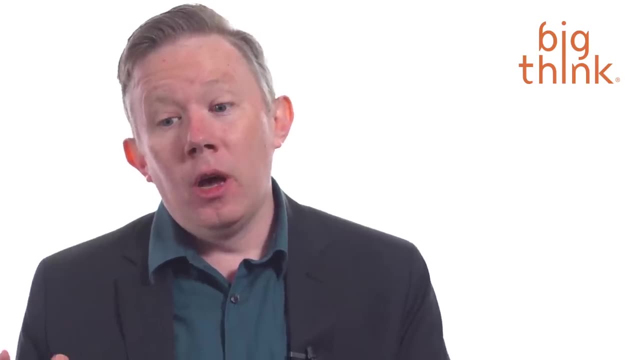 you're not in a zero-sum interaction, you can end up ruining it for everybody, But if you're truly in a zero-sum interaction, this is one of the strategies that you can use. Now, suppose that you're dealing with a—suppose you're dealing with an opponent who's not. 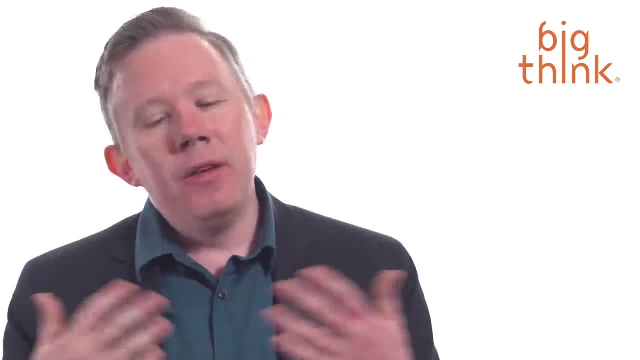 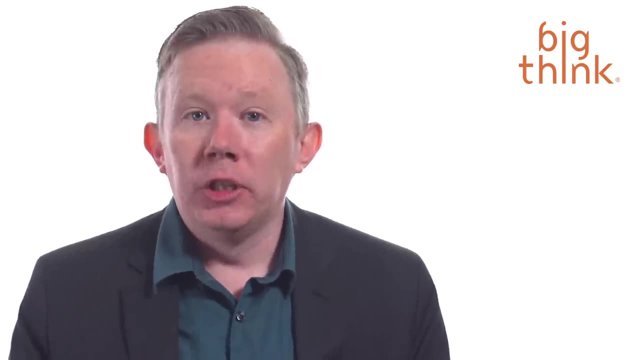 sophisticated, You're smarter than they are There. it depends very much on— How smart are they, Can you out-think them And what's the individual interaction that you're engaged in? So, poker players—to return to the example of poker players- poker players will engage. 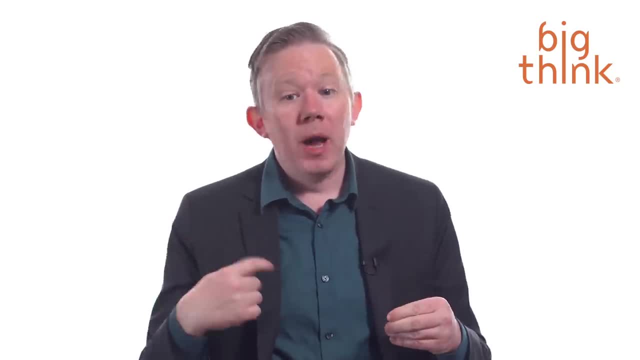 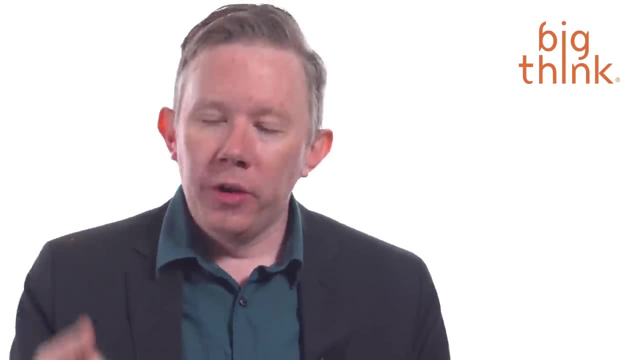 in interactions where they're trying to think: well, does my opponent think I'm going to bluff here? Yes or no? And maybe I'll do the opposite, But that's going to depend on how smart is your opponent. what are they thinking about?